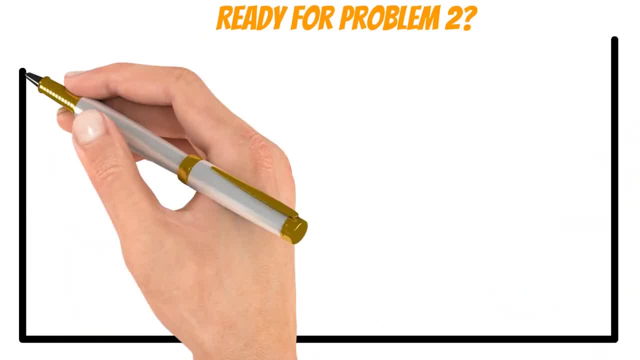 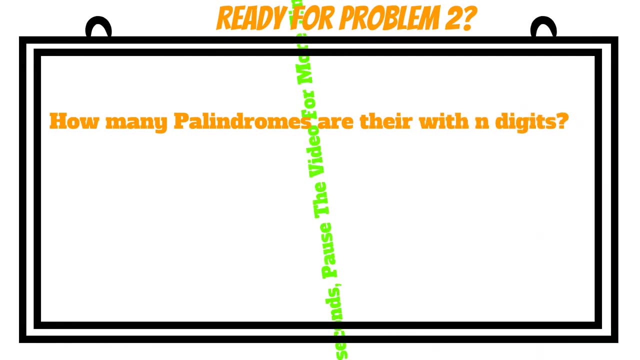 Are you ready for problem 2?? How many palindromes are there with n digits? Your answer should be a formula. You have 30 seconds for this problem. Pause the video if you need more time. Your problem 2 names are the same as your answer. 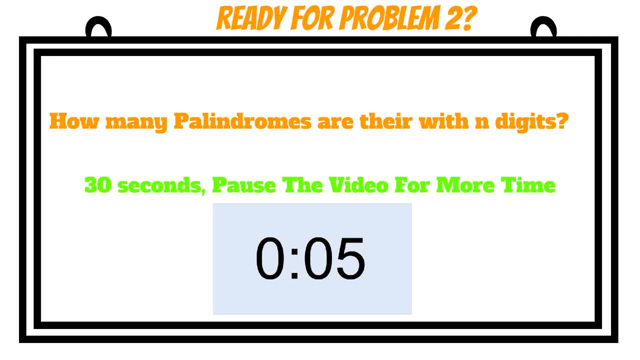 You have 30 seconds for this problem. How do you think your answer is? The correct answer is 2.. Your answer is 3.. It means that 2 palindromes are a positive number or 2 has a negative value. 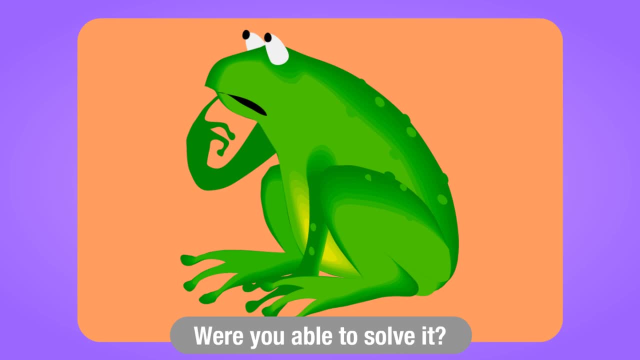 No, that's a false. You can solve it with a problem. So how many three-digit palindromes are there? The right answer is 2.. Who are you? What are you doing here? Answer in 5 seconds. 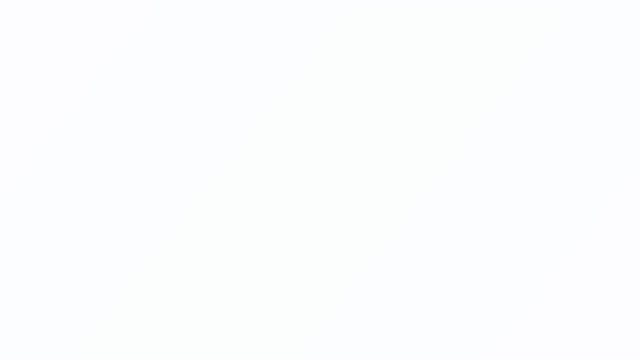 Why would you give me a problem if we don't know that there are three-digit palindromes? Okay, I'm going to go and test them. So here's our answer for this problem. We have two cases: either n is even or n is odd. 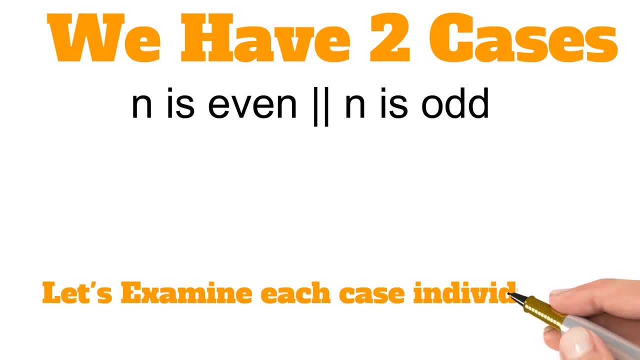 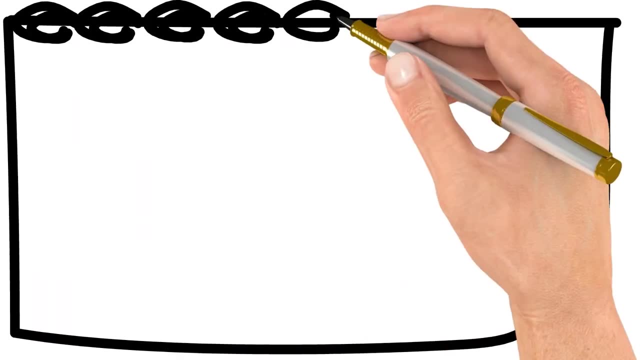 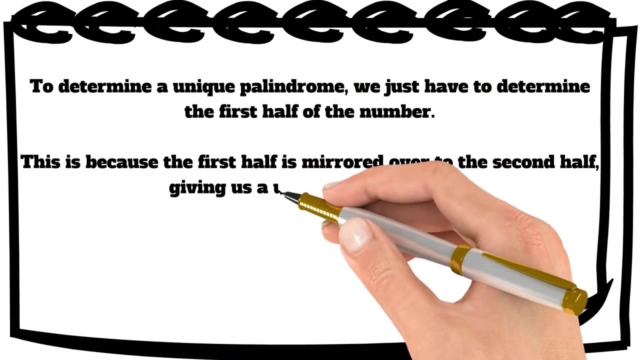 Let's look at both cases. Let's look at case 1, the even numbers. To determine a unique palindrome, we just have to determine the first half of the number. This is because the first half is mirrored over to the second half, giving us a unique. 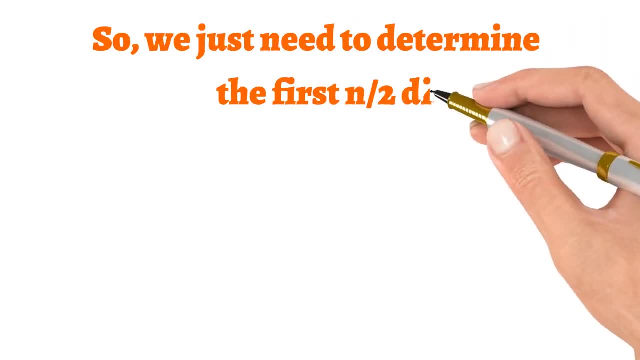 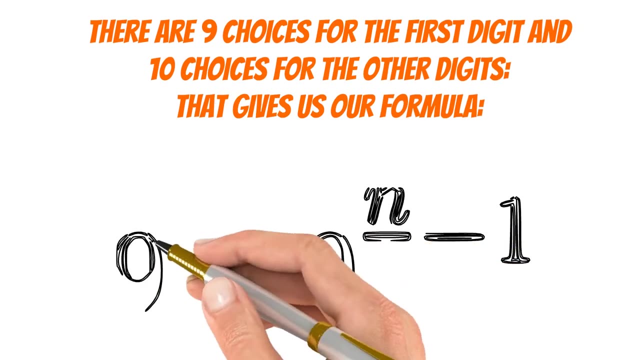 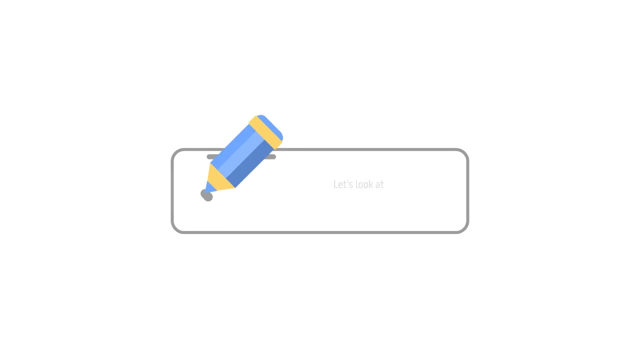 palindrome. That means that we just have to determine the first n over two digits. There are 9 choices for the first digit and 10 choices for the other digits. That gives us our formula. This is similar to the last case. Let's look at case 2 now, the odd numbers. 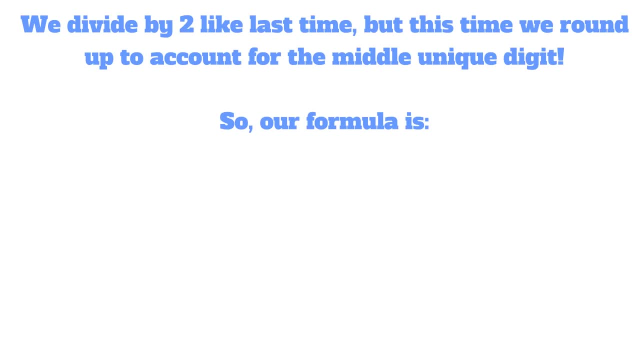 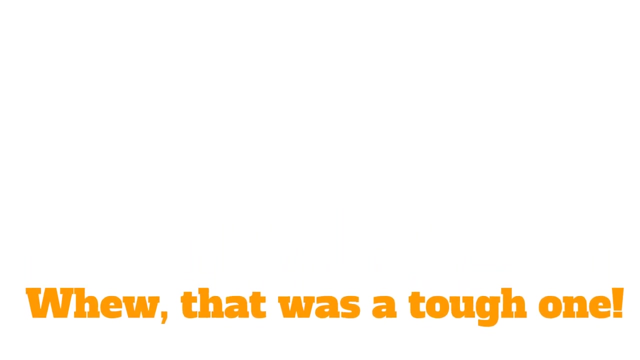 We divide by 2, like last time, but this time we round up to account for the middle unique digit. So our formula is: The last problem was a tough one. Hopefully you learned something about palindromes and I hope that you enjoyed this video.